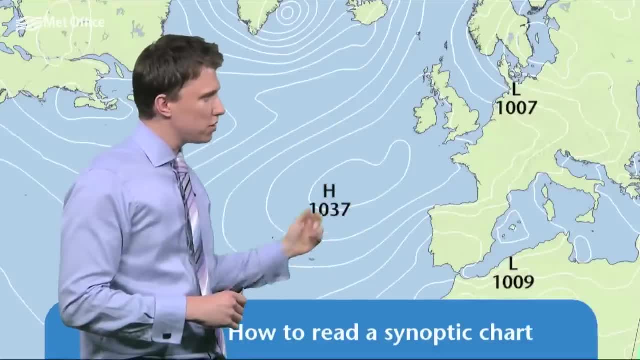 Well, we know that air moves from the north of the chart to the south of the chart, And air moves around areas of high pressure in a clockwise direction and in low pressure in an anti-clockwise direction. So now we know something about the speed of the wind. 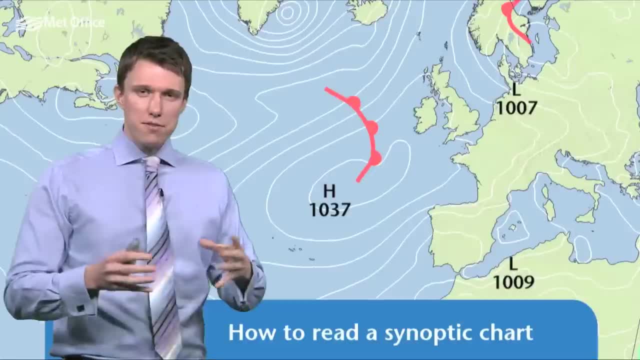 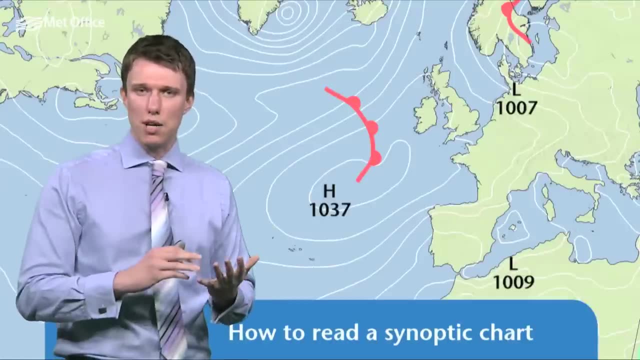 and indeed, where it's coming from. Now, these differences in pressure, temperature and wind circulating around the globe mean that there's different types of air, And by that I mean they have different characteristics, such as how cold or warm they are or how much moisture they're carrying. We need to mark 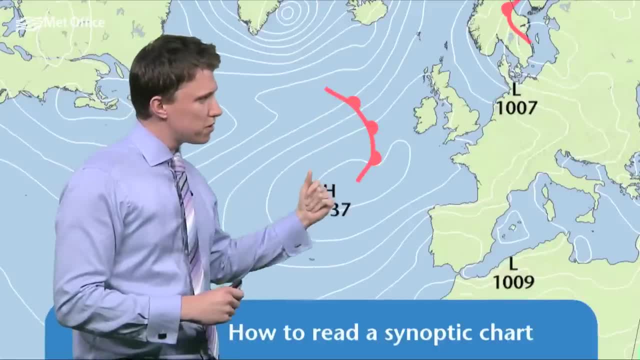 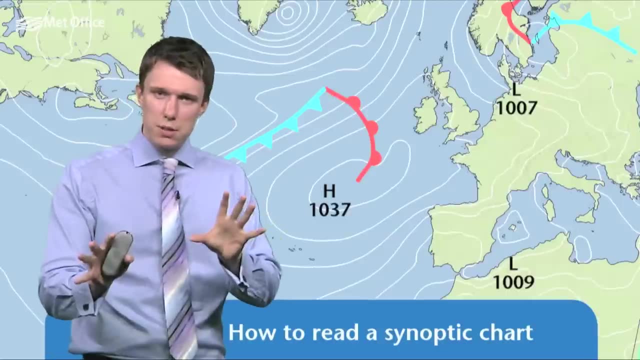 out these differences somehow. So many of you have seen this warm front: It's a red line with red semicircles, and also a cold front, which is a blue line with blue triangles, And these just mark out these differences between how cold and how warm and how moist. 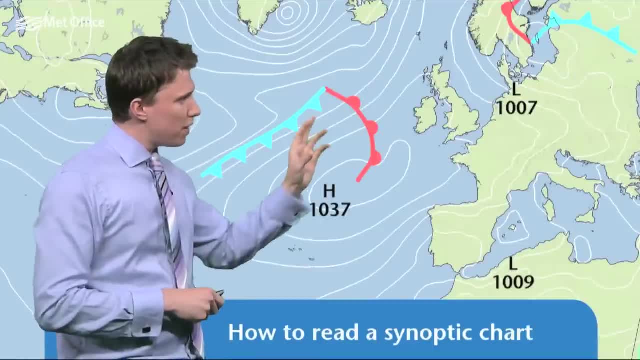 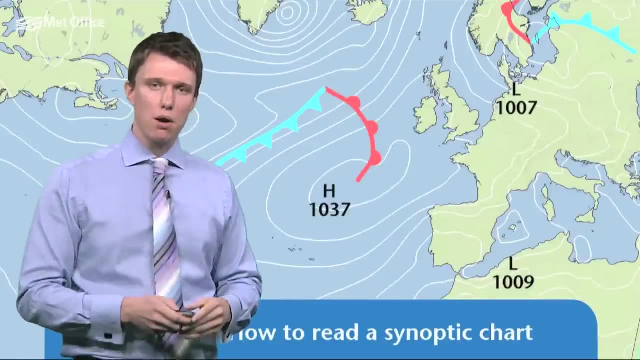 the air mass is And also importantly, we tend to see warmer air following a warm front and colder air following a cold front, And also we see increased amounts of cloud and rainfall in and around the area that the front marks. Another type of weather that you can spot on a weather chart lies between a warm and 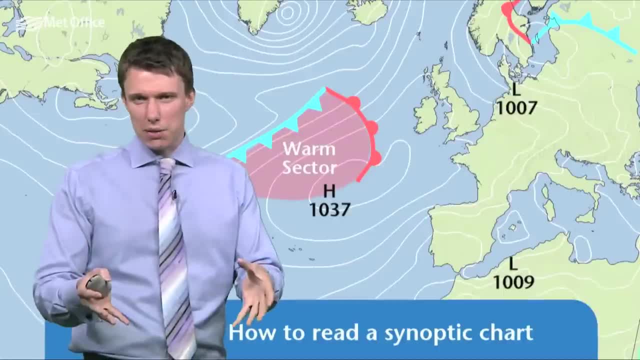 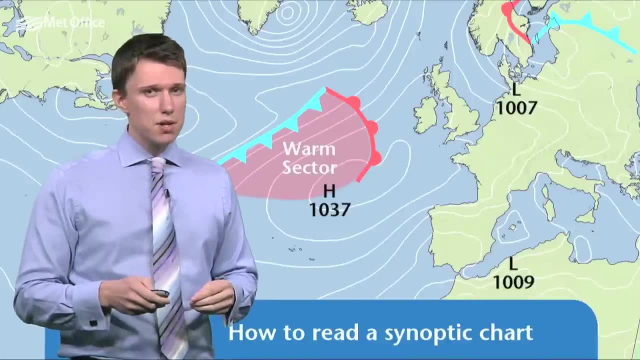 a cold front. That's what we call a warm sector. It's a fairly cloudy type of air mass and it can bring mist and fog and also some outbreaks of patchy light rain from time to time. Now, in time as well, a cold front will tend to catch up with the warm front because it moves. 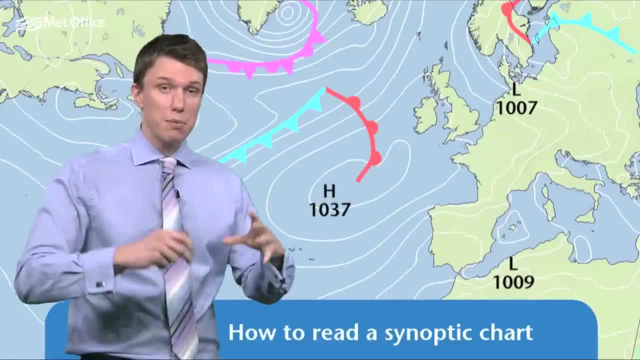 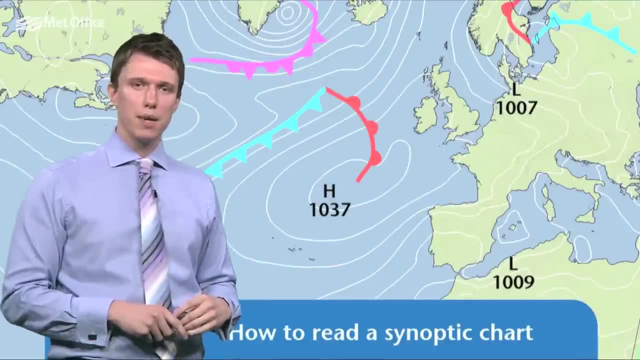 faster and we end up with something called an occluded front. In time, these occlusions can form their own entities as well, But they're marked by a purple line with purple semicircles and purple triangles next to each other. Now, the direction in which these semicircles and triangles point simply marks out the direction. 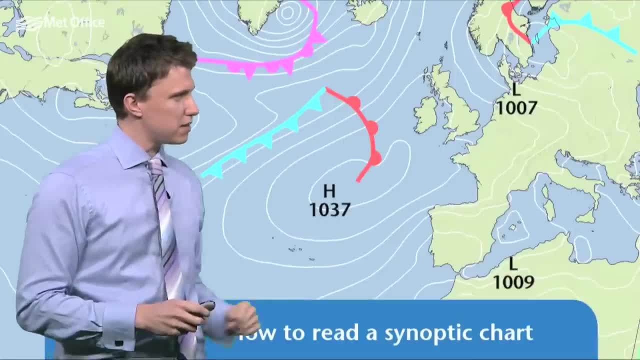 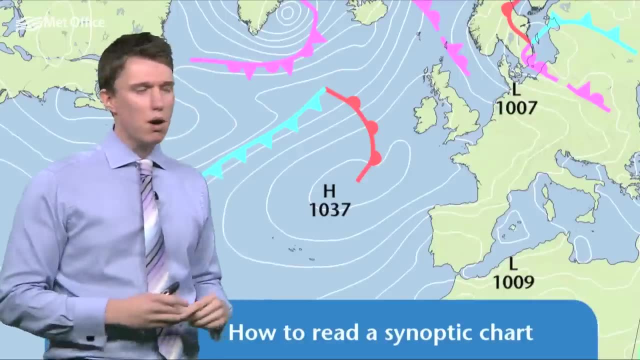 of travel of the front. So we know that these set of fronts are moving from west to east in time. In time as well, this difference between the type of air, how warm, how cold, how moist it is, will tend to become less marked. 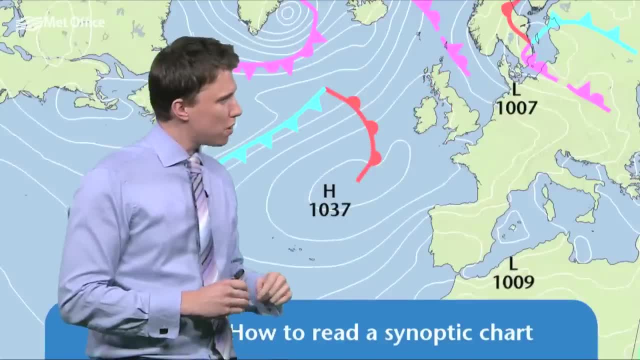 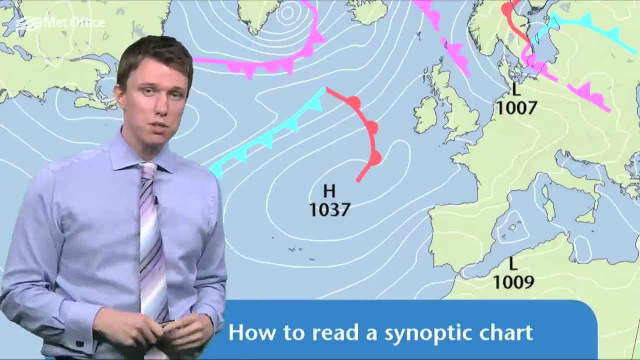 Now you may note that some fronts have a little gap or maybe even a little cross marked in them. There's occlusions there, to the east of the chart, showing that this difference between the air is weakening. They're called frontalitic fronts And sometimes you may 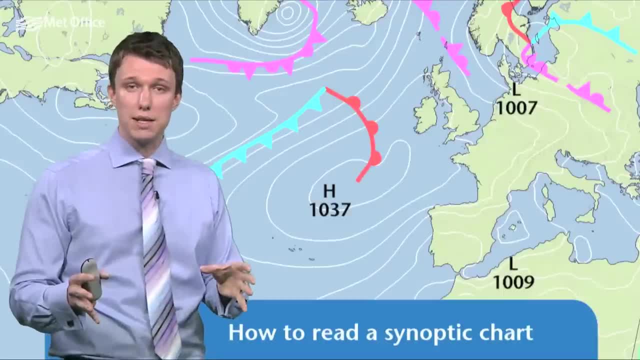 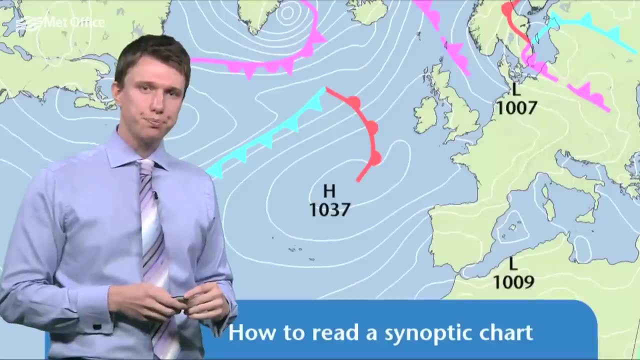 also see a set of fronts which have the triangles and semicircles that are unshaded, And these are what we call upper fronts. They're the same as the fronts at the surface, but they mark differences in the air higher up in the atmosphere.